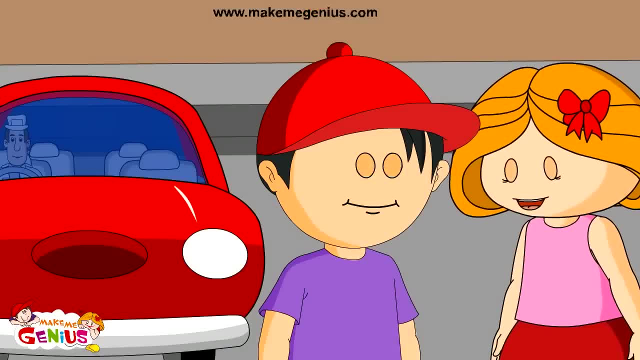 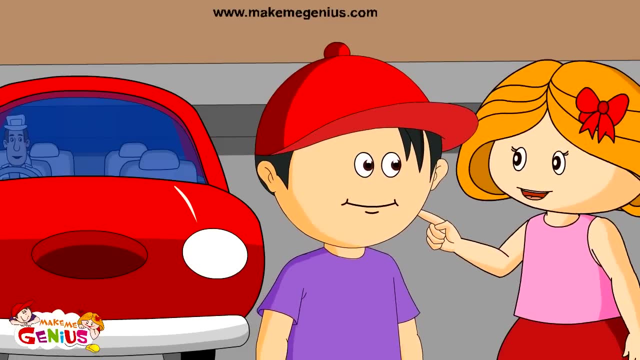 let me go now. we are in love with the car. let us go to thekers. grey, we are going to come and join you in the backseat, Jimmy. one more rule: you should always come in or out of the car from the curbside of the road. okay, okay, let me come from this. 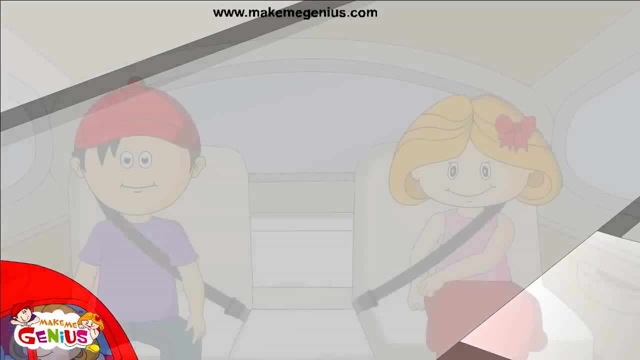 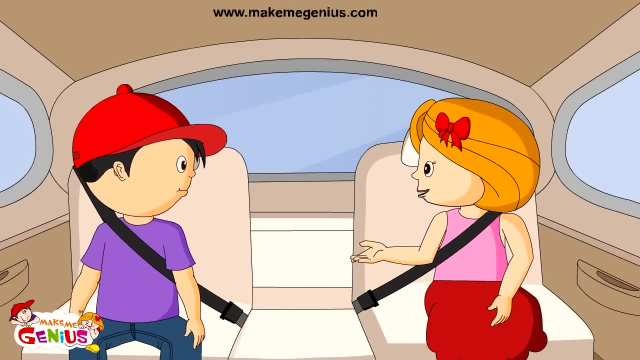 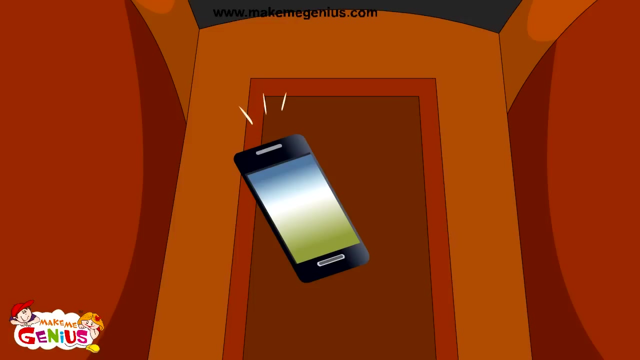 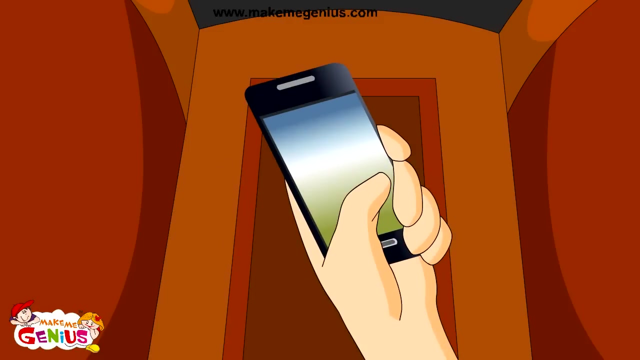 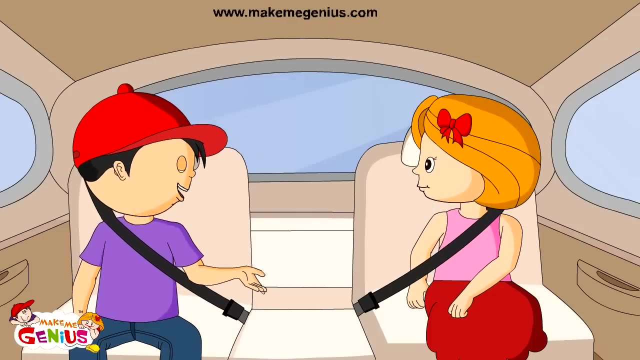 side. tell me, why should we wear seat belts? we should always wear seat belt and sometimes drivers apply brakes suddenly. if you're not wearing a seat belt, the you may hit your head on something and that can be dangerous. why did you ask uncle to not answer his phone? because we should not talk on our mobile phones. 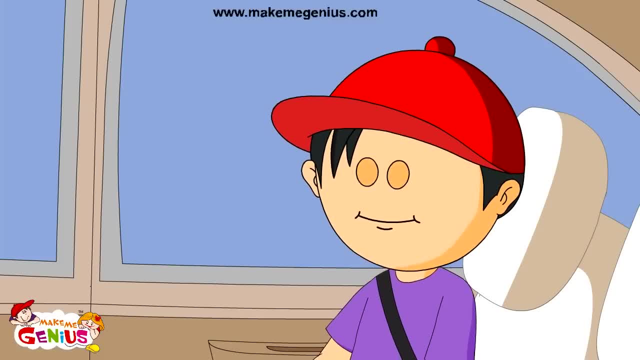 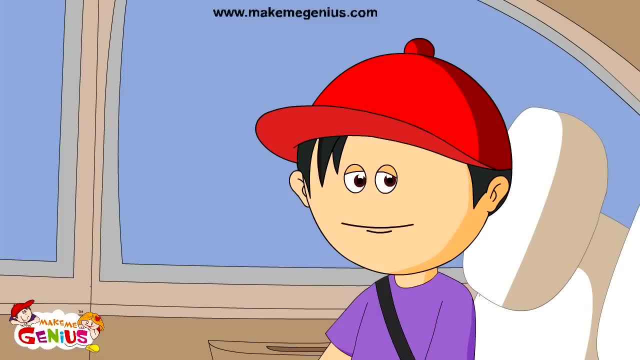 while driving. it can be very dangerous. while talking on our phones we don't pay full attention to the road. it can cause an accident. oh, I will tell this to my school bus driver. he is always talking on his cell phone while driving. look, the signal is now red. our car is. 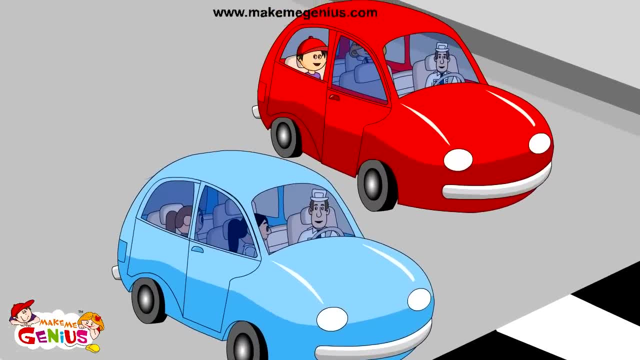 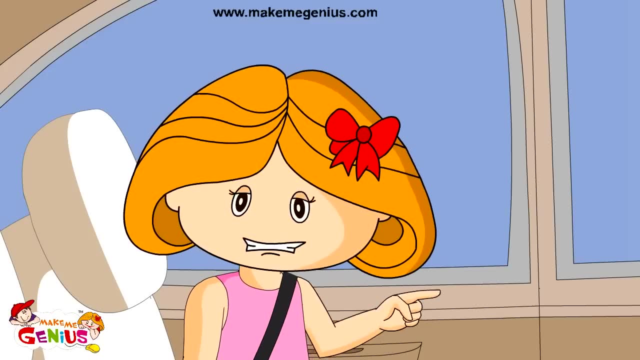 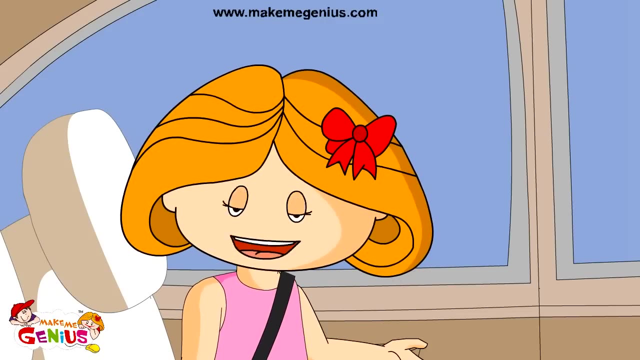 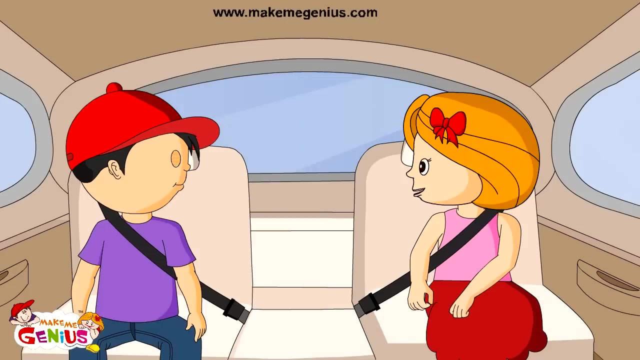 slowly stopping. hey look, it's my friend in that car. let me say hello to him. Jimmy, that is dangerous. you should not take your hand or head out of the car on the road. if another car or a vehicle is coming from behind, it can hit you. oh, I am so sorry. I never thought like that we. 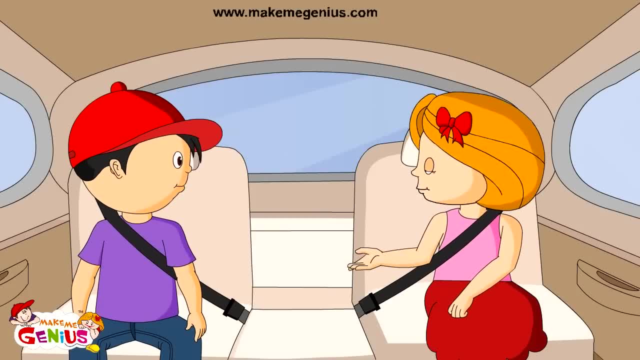 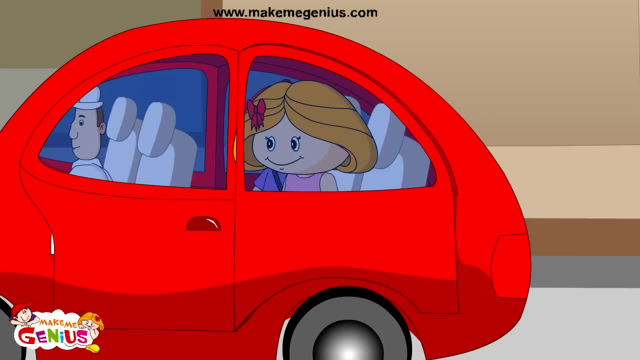 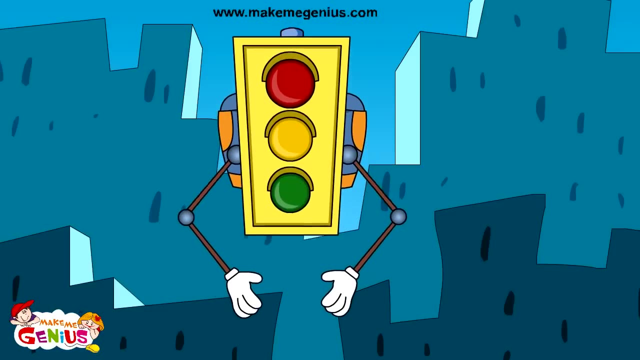 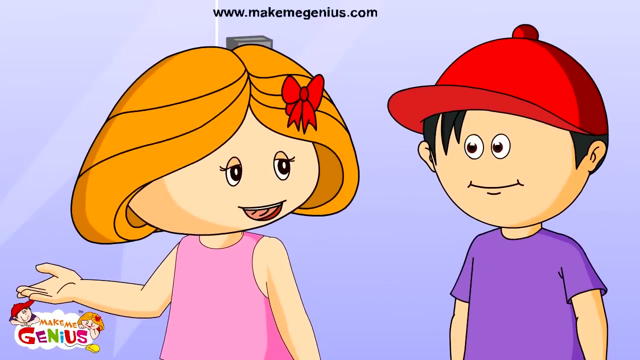 have to go to the market area, let's go outside. remember the rule: we should always get in or out of the car from the curbside of the road. oh see, our friend is here too. hmm, yes, traffic lights are our friends. they help in controlling the traffic, hey. 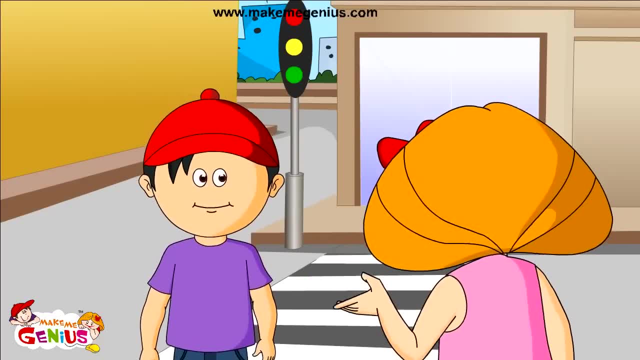 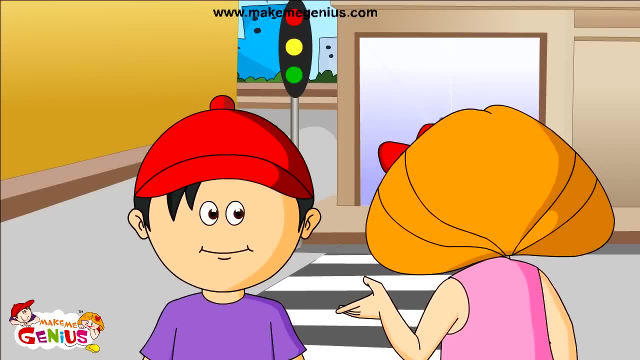 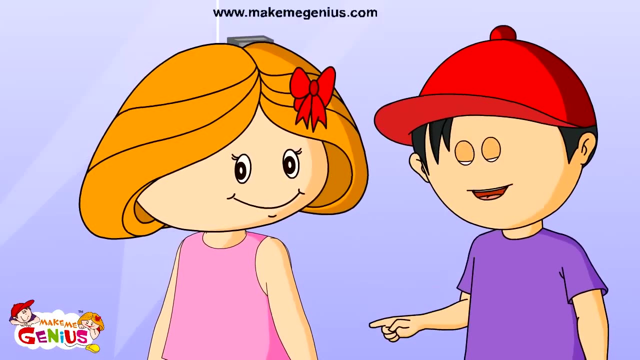 stop. did you see the signal? it is still green for the traffic. we should cross the road only when the signal for the vehicle is red. oh sorry, and I'm also not. one rule: we should always cross the road from pedestrian road. perfect, we can drive here only for driving girl flavors. you got it. 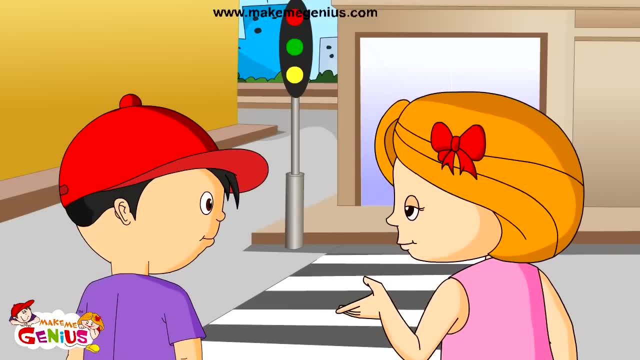 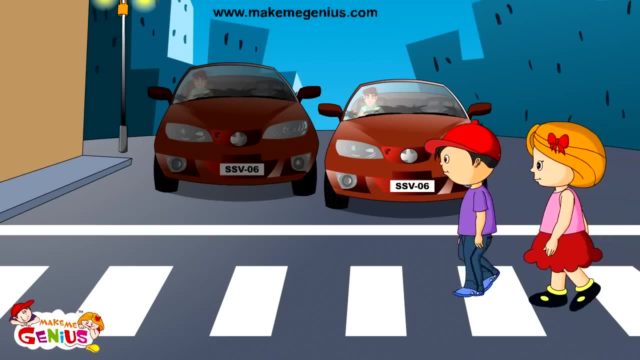 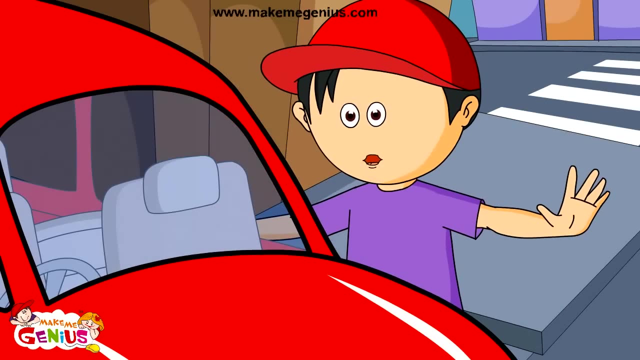 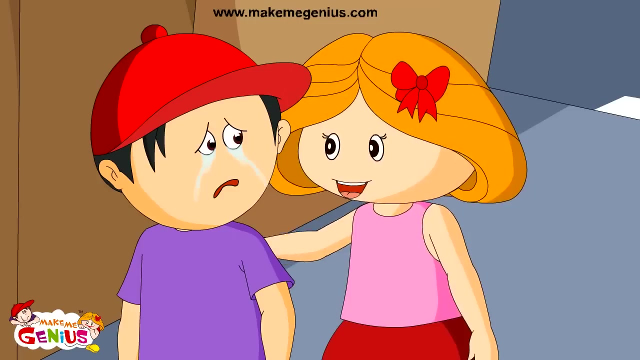 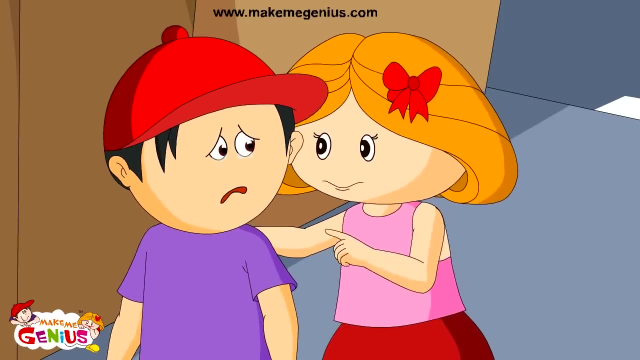 crossing he. yes, it's also called zebra crossing. see, now the light has gone red for the traffic. now we can cross the road. oh, that was very close. don't cry, nothing has happened, you are safe. but remember, don't run or play while you are on the pavement. it can be very dangerous. I will 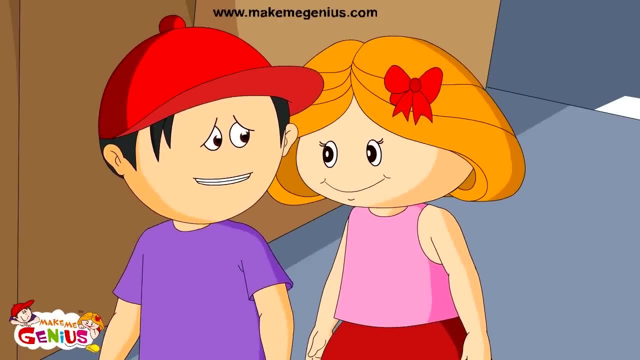 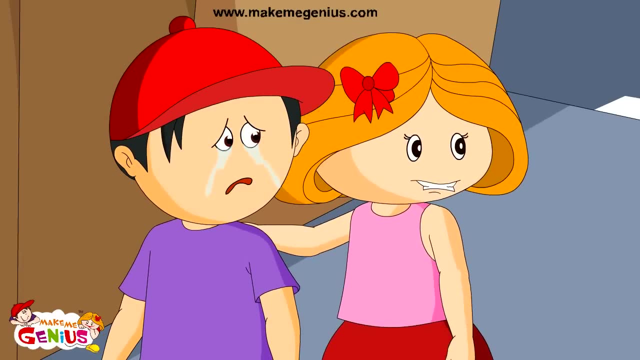 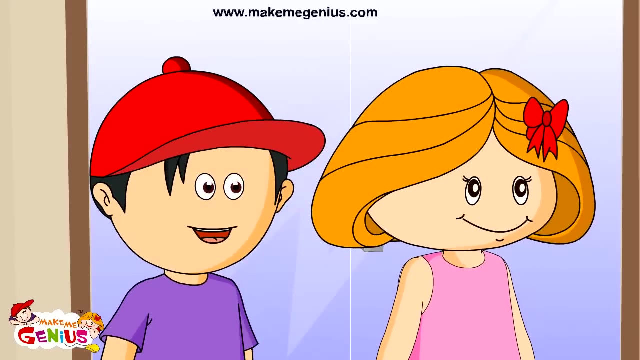 take care next time. pavement is for walking, it's not for playing. you are very intelligent. oh, let's go to the other side, but we can't cross the road as the signal for pedestrians is red. let's wait, it's green now, but before crossing we should look both. 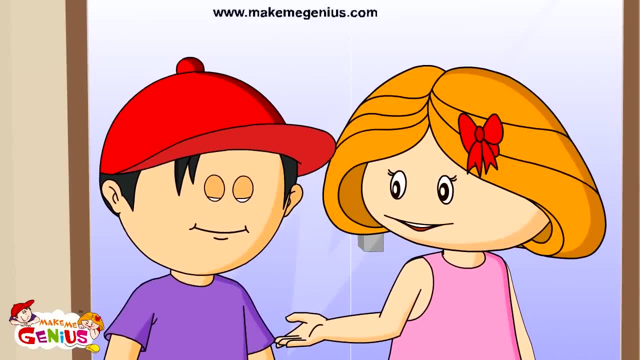 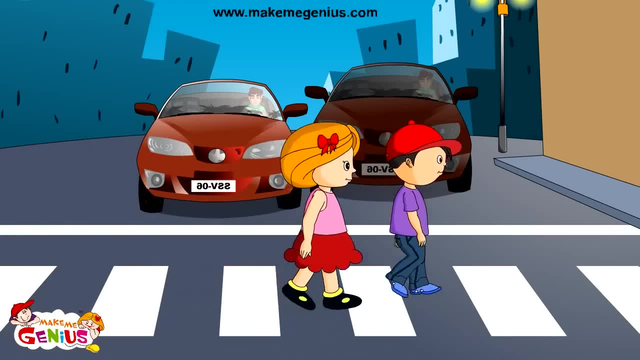 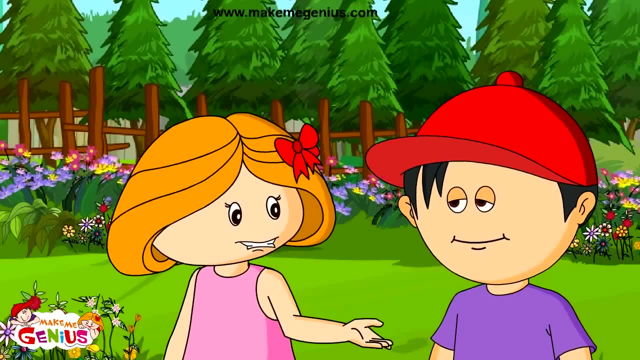 ways to make sure that we don't get caught in the traffic jams. but before crossing we should look both ways to make sure that we don't get caught in the traffic jams. sure that all vehicles have stopped? now we can cross. Wow, it's a park. yes, here we can learn about traffic signals. let's go to each. 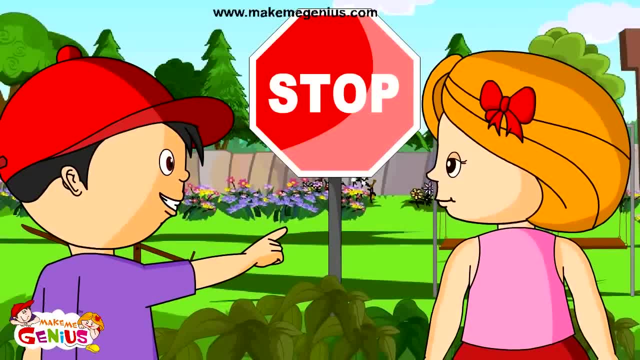 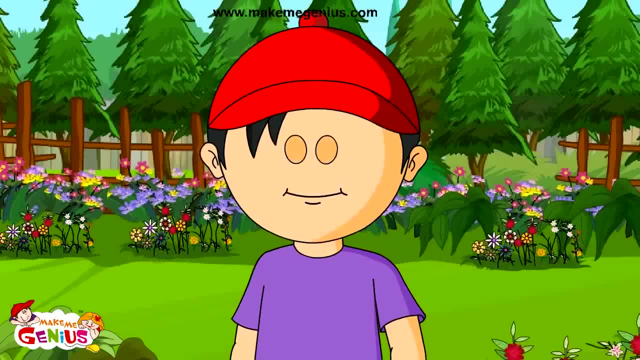 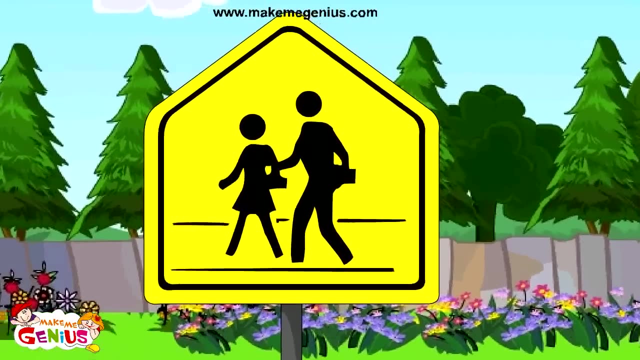 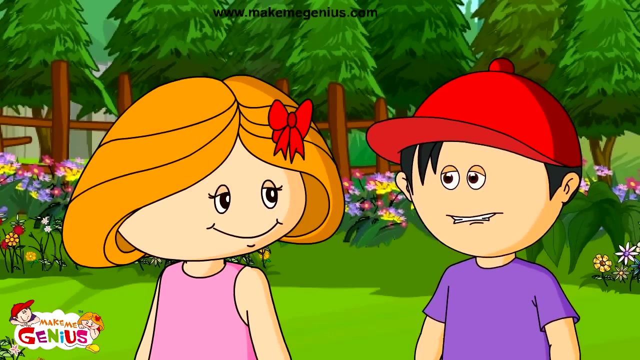 one. it is written stop. what does it mean? it means we should stop and look for other vehicles. there is no other traffic, then we can move. let's go to the next. I know about it. it is near to my school. it means that you are near school and you should slow. 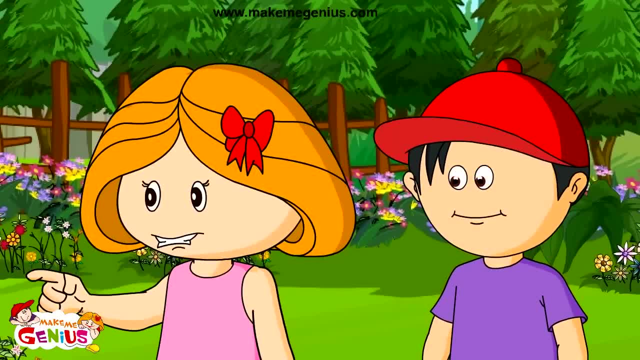 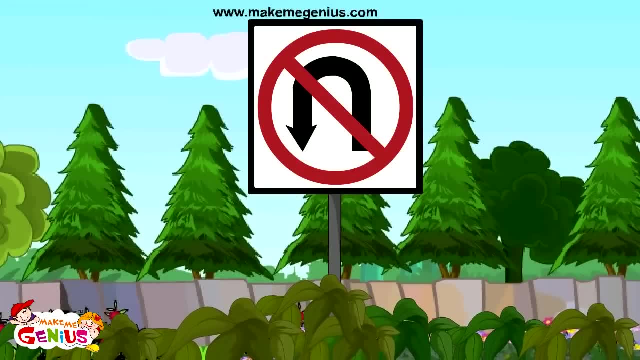 down. you are right. look at this sign. it's means you can't take a left turn. what is this sign? oh this. this tells you you can't take a left turn. What does this sign mean? oh this, This tells you you can't take a left turn. 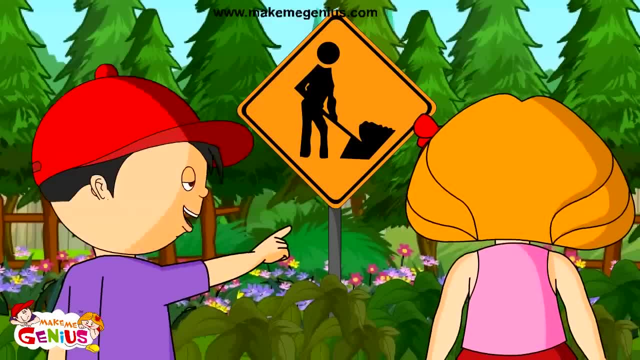 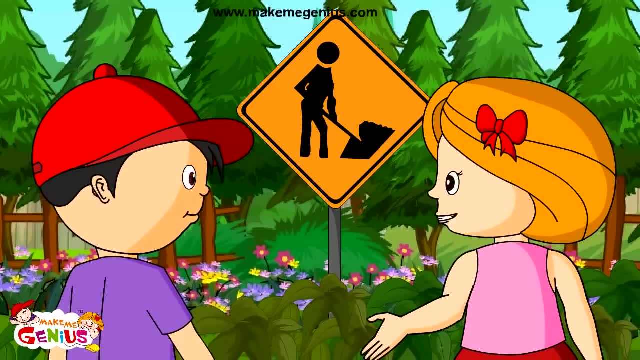 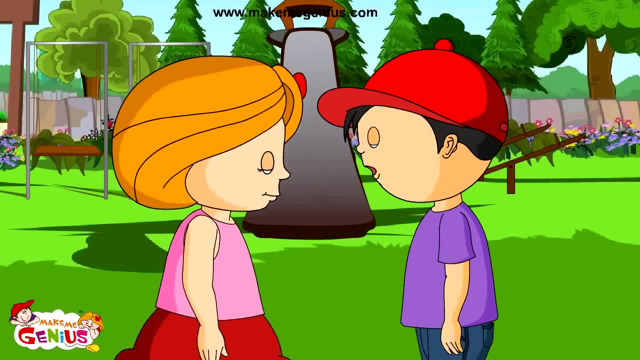 you that we can't take a U-turn from here? Look at this sign. It seems some person is walking. You are right. This sign tells you that there is some work going on, So either we should be slow or we should take another route. Thank you, Ginny. I learned a lot today.